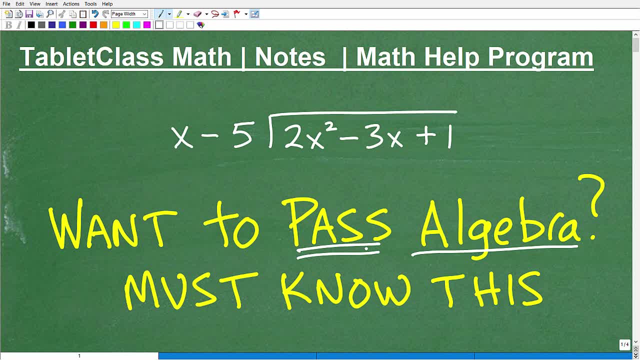 so I'm talking about, like Algebra 2, College Algebra, Intermediate Algebra. this becomes even more important. But this is really an interesting thing that we're going to be talking about here, because there's a connection to what you were doing way back in the good old days when you were in like the third grade, fourth grade, and you were doing arithmetic. 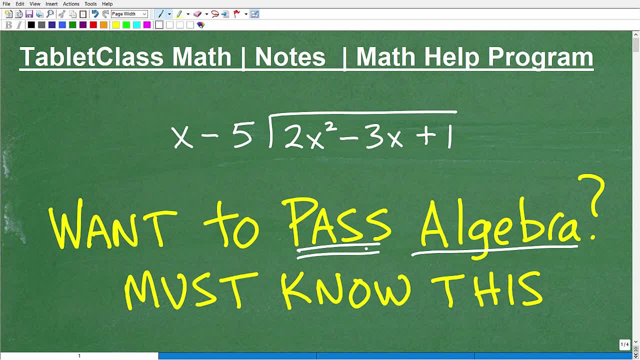 And probably a lot of you were thinking: well, when I do arithmetic, I'm working with just basic numbers. You know that's like one math. and then when I take algebra, that's like a completely different math. But no math is connected. all right, It's. you know, it's all like one big bucket of mathematics. 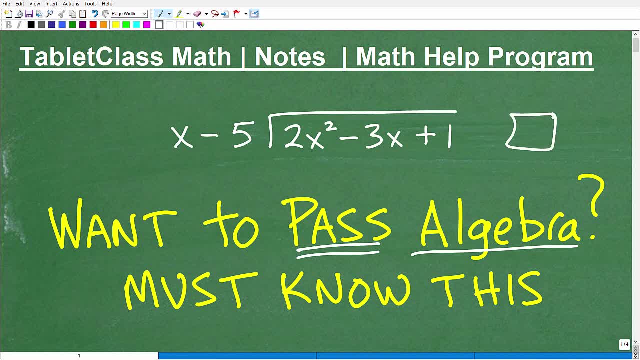 It's not like you know. you do arithmetic over here and that's like the only thing you do. It has nothing to do with algebra. That is not the case at all, and you're going to see this in this particular video. 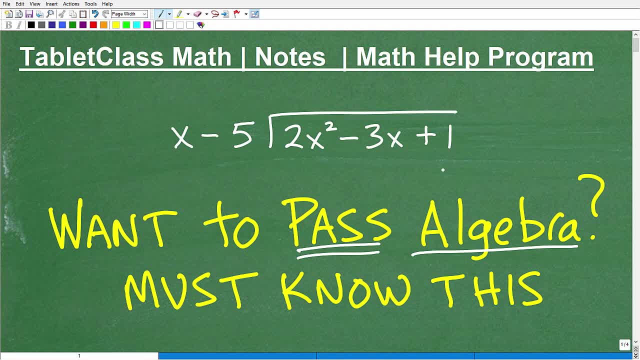 What we're talking about is polynomial long division. okay, So we're dividing. Now, this is interesting, You might like. well, could we use this division symbol? Yes, we could use that division symbol to represent this. but there's, you know, I have this little thing right here. 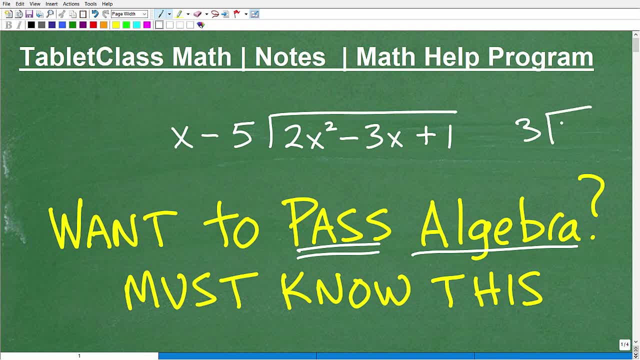 As you may recognize from problems like, say, 3 goes into 42,. all right, This is exactly what we're going to be doing here. So, yeah, If you never heard of polynomial long division, this would be a good introduction to it. 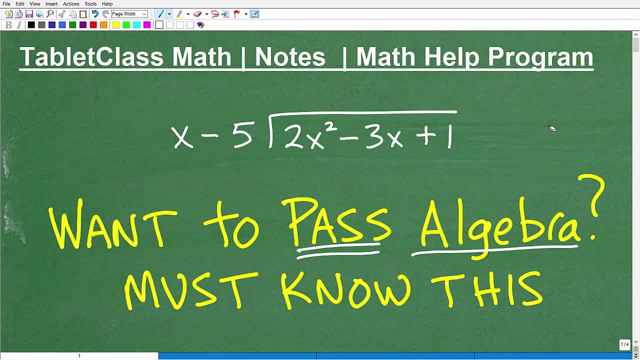 and not only am I going to show you polynomial long division, I'm going to show you a shortcut method that we can use sometimes with polynomial long division. You absolutely need to know It's super cool. It's called synthetic division, So we're going to talk about that as well. 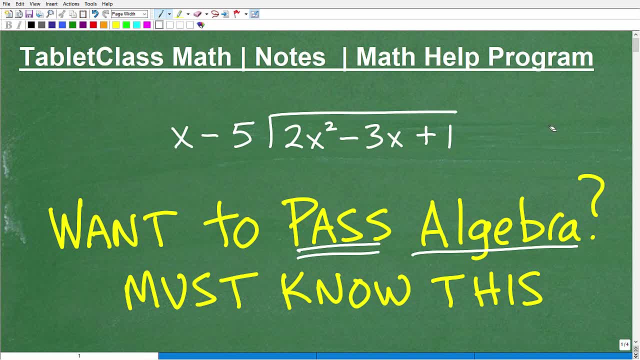 So, again, this is just a quick introduction to polynomial division in general, but you absolutely need to know this to be successful in algebra. So we're going to get into this In just one second, but first let me quickly introduce myself. 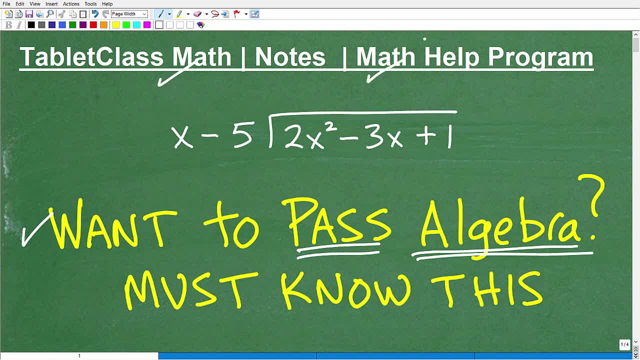 My name is John. I'm the founder of Tablet Class Math. I'm also a middle and high school math teacher and I've been teaching for decades. all right, And along that time I kind of felt the passion to create something special for my students. 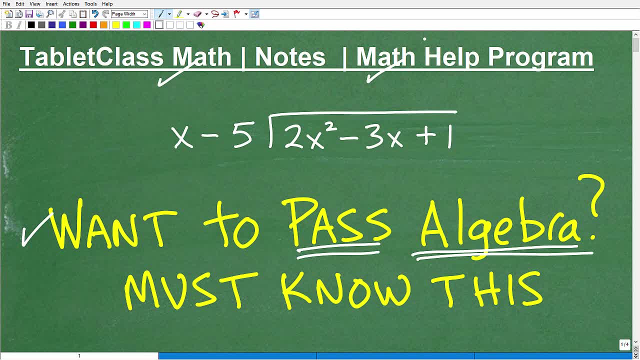 So I've created what I like to believe is one of the best math help programs there is. I've been working on my math courses and my math help program for 15 plus years, Very proud of it because I've put a lot of effort. 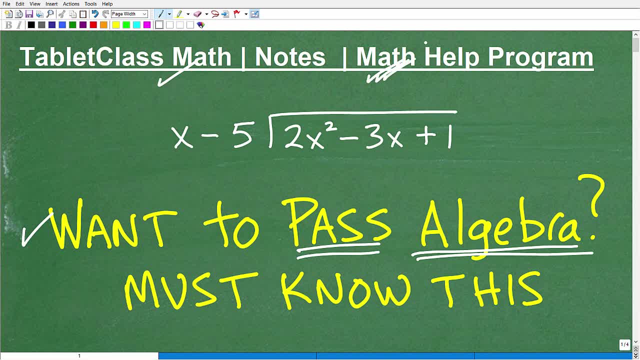 I've put a lot of effort into it but effectively I have 100 plus different math courses, ranging from pre-algebra, algebra 1, geometry, algebra 2, finishing up with pre-calculus. We'll have that out in a couple weeks. 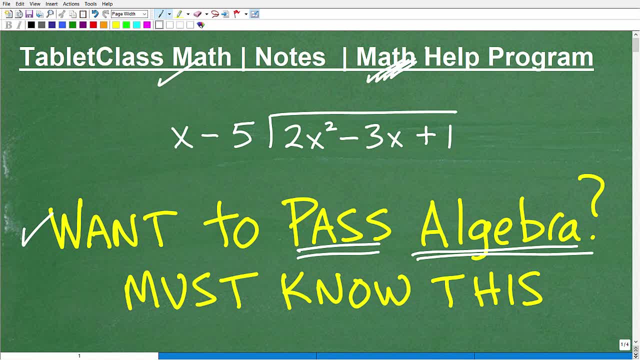 But I also do a lot in the area of test preparation. So if you're studying for an exam like the GED, HiSET, TASC, SAT, ACT, GRE, GMAT, ASVAB, CLEP exam, ACCUPLACER, ALEKS, a teacher certification exam, nursing school entrance exam, like the TAS, 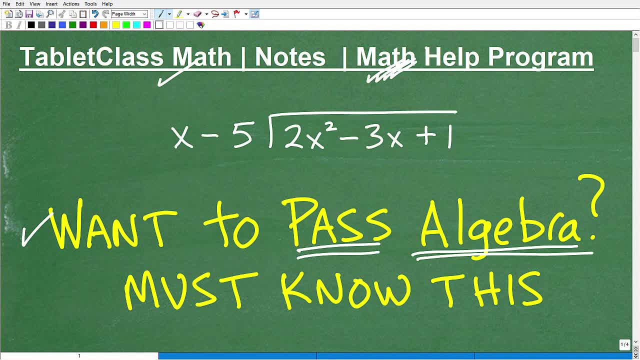 there's so many exams out there that people have to take, And all these exams have math on them. So if you don't do well in the math section, you don't do well on the exam. I could definitely help you out Again. just go to my website. 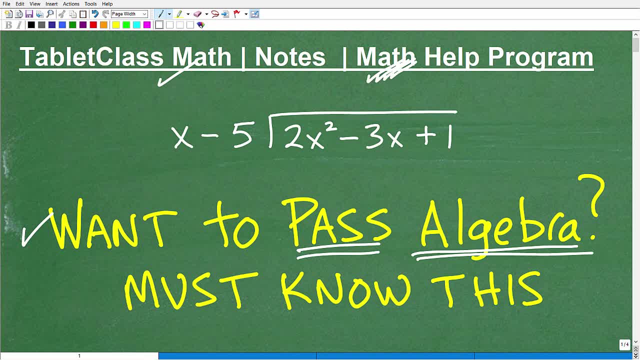 The link is in the description of this video and check out my full course catalog. By the way, if I don't have your exam, drop me a line and I will help you out the best I can. I also do a lot with independent learners, like homeschoolers. 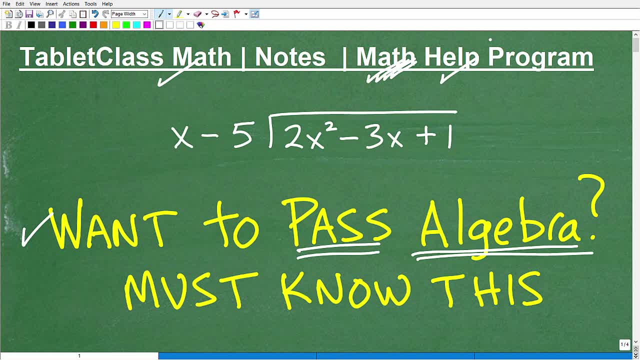 So if you homeschool, I have a great homeschool learning program- And then obviously help those of you that are just struggling in your current math courses. Now, if you're truly serious about wanting to improve in math, if you're like looking for shortcuts, 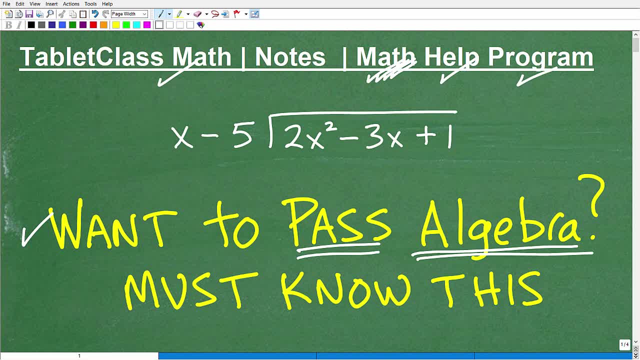 well, I have a few shortcuts in math, But you know, I would say shortcuts will help you about 1% in mathematics, because there really isn't any shortcuts. What you got to do is you got to work hard at learning the subject. 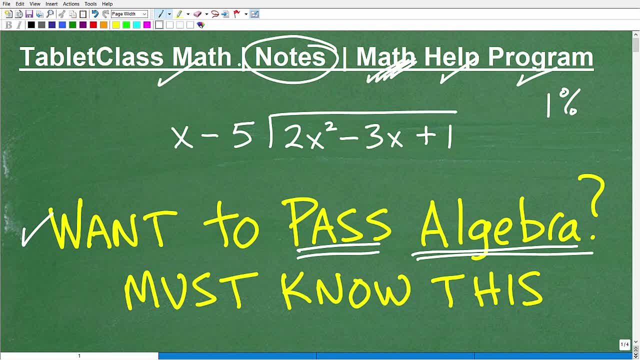 OK, so it all starts with note taking. Now, I've been teaching mathematics for decades and it's apparent to me that those students who take great math notes, they just always do very, very, very well, And the reverse is true. 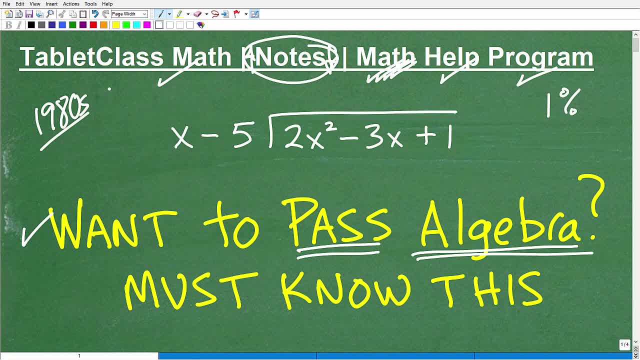 Those things were like me way back in the good old 1980s. which, what was I doing? Well, I certainly wasn't taking notes. I was taking notes, but I was writing to my friends saying, hey, what are we doing this weekend? et cetera, et cetera. 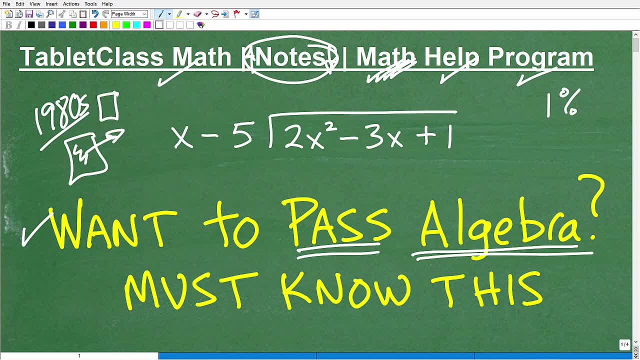 So, listen, I was distracted. I can't even imagine having a cell phone back in those days, because I may not even have graduated high school. Who knows, I wouldn't be making these videos because I wouldn't have gone to college, et cetera. 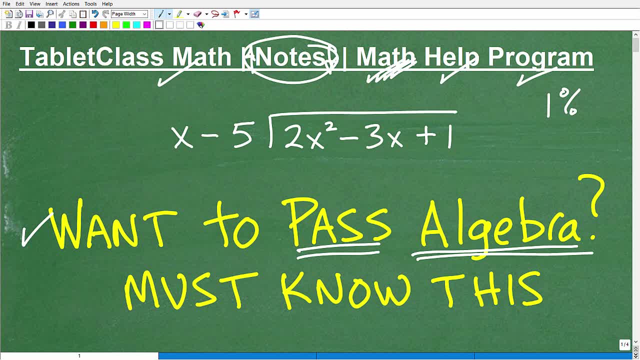 So I get it that you are completely distracted. That's just the way things are. OK. however, you're going to have to have the self-discipline and focus to pay attention to what the teacher is saying and write things down. I'm sorry. 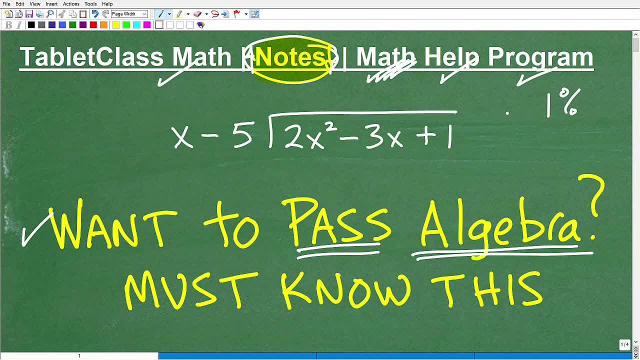 There is no other way than putting in the daily work to take great math notes. but it will pay off. OK, so take great math notes, End of story Now. in the meantime, you still need something to study from for all the things they may have missed. 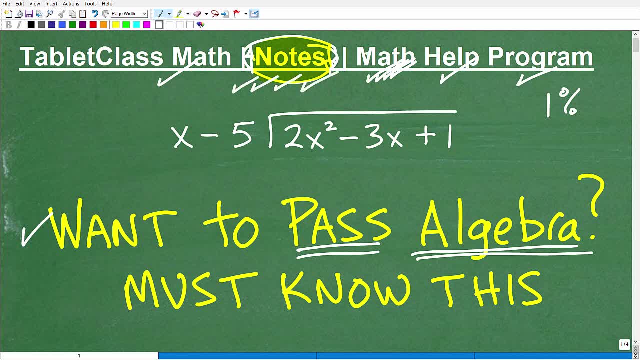 So you can use my math notes to include pre-algebra, Algebra one, geometry, algebra two and trigonometry. You can find the links to those notes in the description of this video as well. All right, Now we're going to get into this polynomial division. 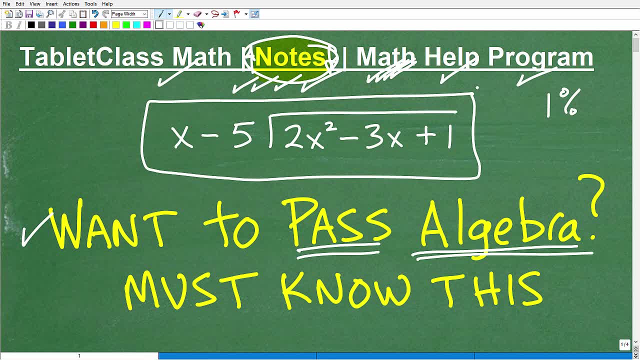 This may be a little confusing for you. This isn't going to be a full lesson on this, but I'm going to demonstrate this problem here And I'm also going to do the same problem using that division, just to make this- you know- impression upon you of how important this is. 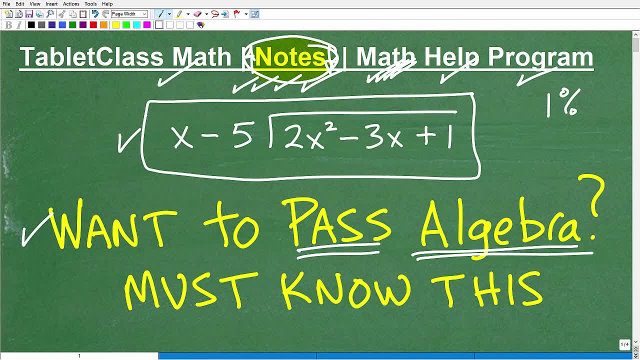 OK, now, if you think you can do this, Definitely pause video and you know, see what you come up with Now. if you need more additional help beyond this video, I do have other videos on polynomial division in my YouTube channel, in my Algebra 2 playlist. 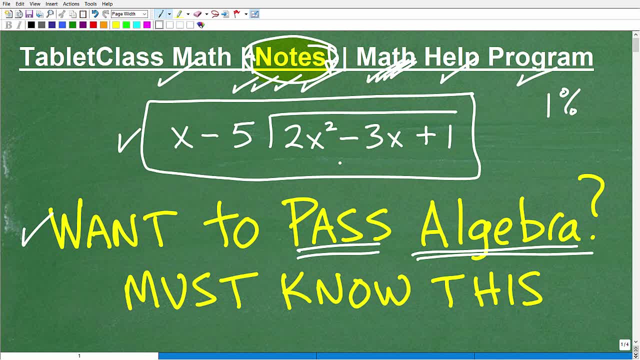 However, you're probably you really want to consider taking like my Algebra 2 course, because I really thoroughly get into this. So this video is just going to be a quick review on this, but not anywhere near the level of instruction I do in my math help program. 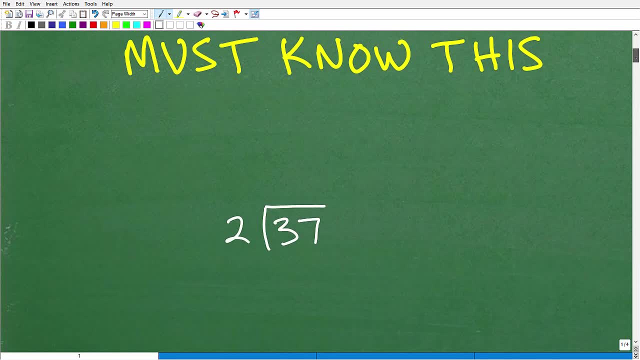 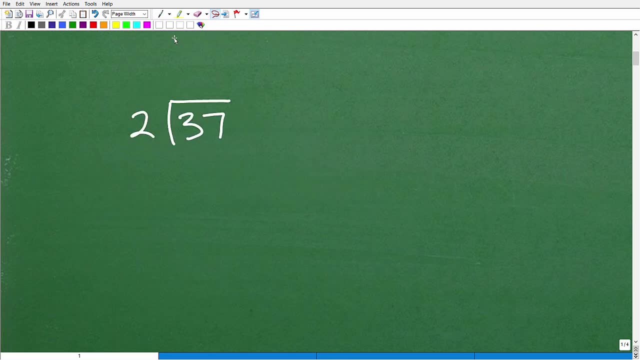 So let's go ahead and get started, And we're going to start first by going down memory lane and doing this problem. OK, do you remember this problem or problems like this way back when you were like in third grade, when we had recess? 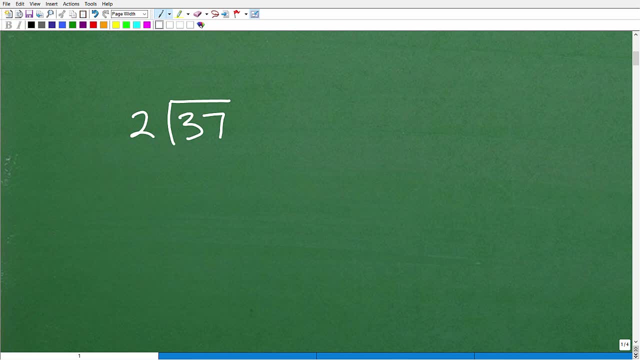 Right, How cool is recess. I wish I had recess. They should make that a law that even adults can have recess. But anyways, let's see if you can do this problem here. Do you remember how to do a problem like this? 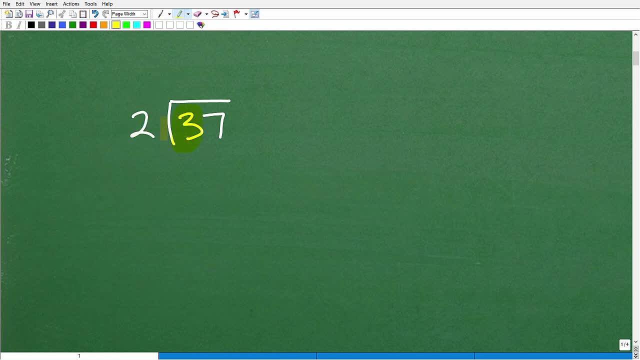 All right. So what do we do? We're like, OK, we got to can to go into three. Yes, Two goes into three One time. Now, hopefully you were taught division something like how I'm doing it. I know there's newer ways of doing division, et cetera. 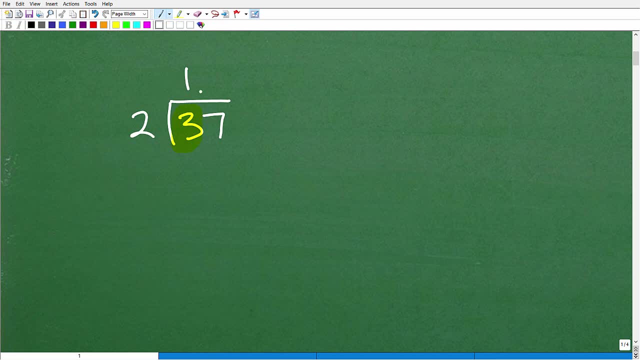 I'm not going to get into comedy on that, But listen, the bottom line is you still need to be able to do this arithmetic, So let's go ahead and continue on. This is the way I was taught way back in the good old 1970s. 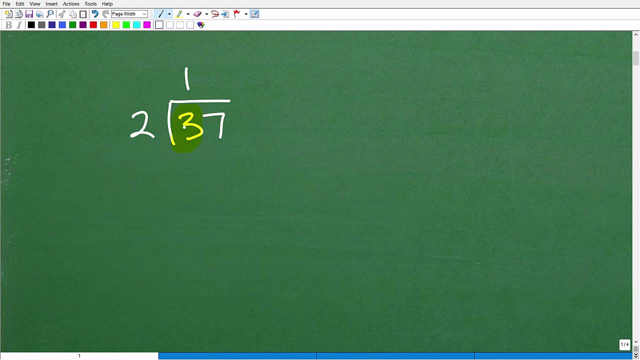 I think my one of my teachers was named as Mrs Pete. All I know is that she was smoking in the classroom. I think that was like 1975.. Anyways, let's get back Back to the problem. So two goes into three. 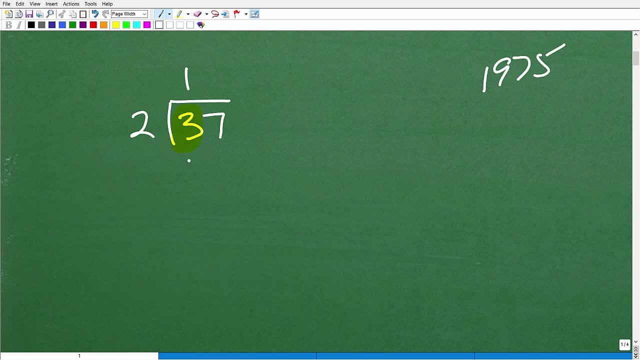 How many times One? So then we go: OK, one times two is two. And then we subtract Right, And I subtract, I'm like: oh, the answer is one, Then I go: all right, can to go into one. 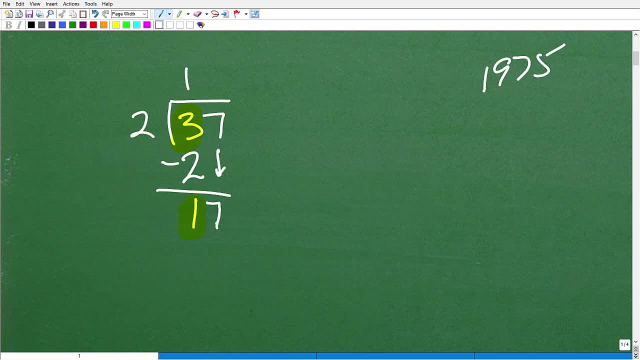 No, it cannot. So I'm going to drop down that seven and I'm like: OK, two can go on to 17.. How many times? I think eight times. Then I go eight times to that 16.. Then I'm going to subtract. 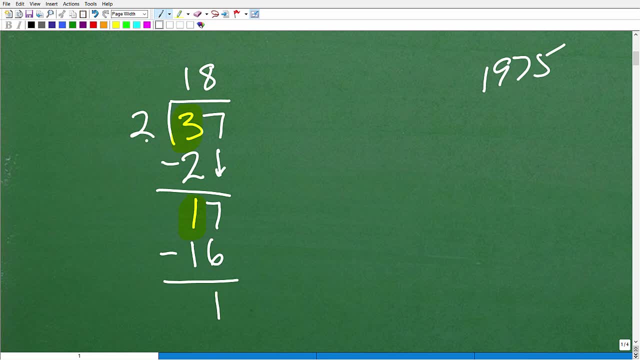 OK, just like I did right here, And then I end up with one Can to go into one. No, but I don't have any other numbers to drop down, So I'm done. So I can say: two goes into thirty seven, 18.. 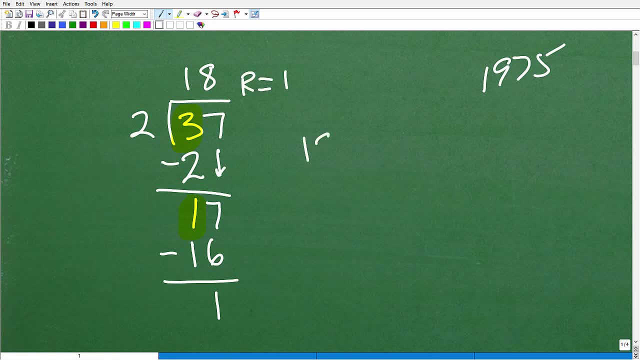 Remainder is one, or I could go 18, and I could write this as 18 and one half as well. So hopefully most of you out there remember this, because this is called the division division algorithm. All right, This is very, very important in even advanced mathematics in an algorithm. 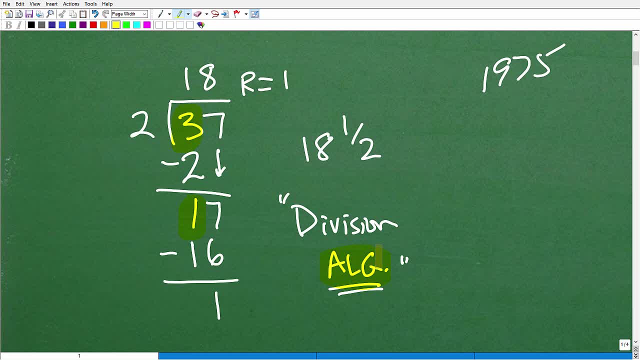 If you don't know that it's basically a computer program. a computer program, Yeah, that's pretty much. it Like a recipe, It's a step they follow. OK, it's like you know, when I want to do division, I run this computer program. 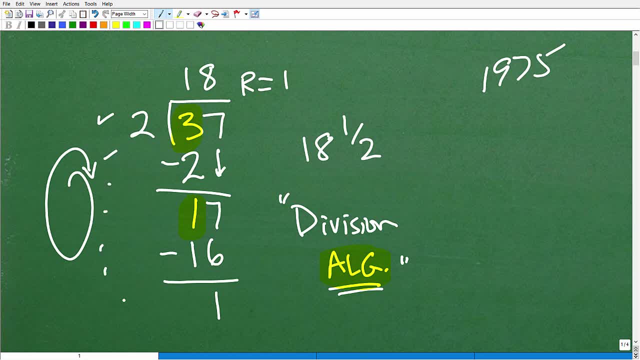 I do these steps: that, that, that, that, that. So that's what you were taught. You may not know your teacher. I'm sure your teacher, like my teacher, wasn't say: today we're going to learn the division algorithm. You start learning division and you naturally kind of just follow these steps. 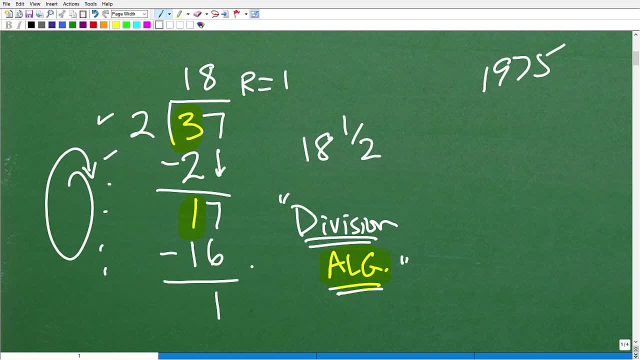 Well, we're going to apply these steps here when we're dividing polynomials. All right, But now let me kind of just quickly tell you why this is so important. Like, why do we even care about dividing polynomials? We're taking one polynomial and we're dividing it into another polynomial. 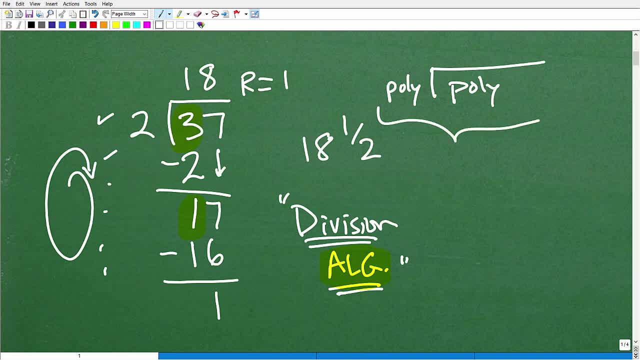 What's this even all about? Well, this skill- what we're doing is kind of a core skill Set to solve: solve advanced, advanced polynomial equations. This is really what this is talking about. This is the skill that you need to solve an advanced polynomial equation. 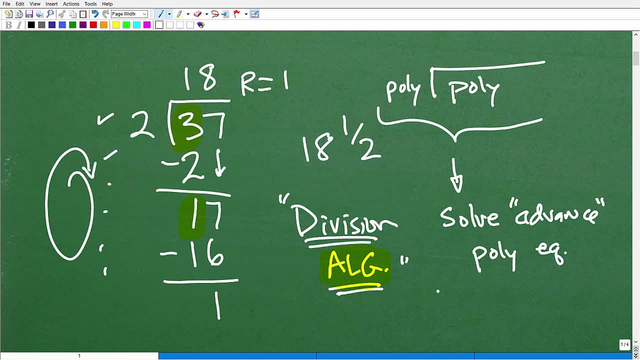 Now I use the word advanced because I'm talking about any polynomial over a second degree, above a quadratic equation. So if I'm saying, solve, solve this, This polynomial equation, all right, I'm just going to make something up here. So here's a polynomial equation. 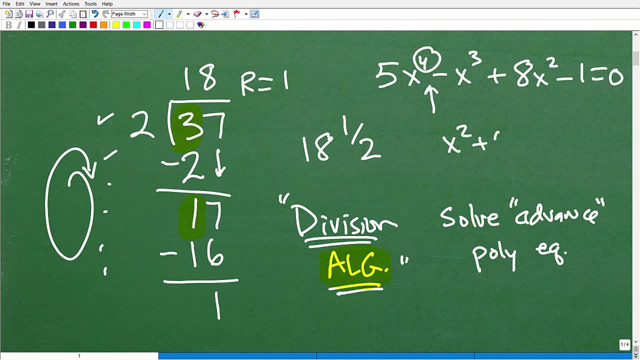 It's degree four. If this is degree two, like x squared plus six, x minus eight is equal to zero. Well, hopefully most of you will recognize this is a quadratic equation And there's all kinds of ways that we can solve quadratic equations. 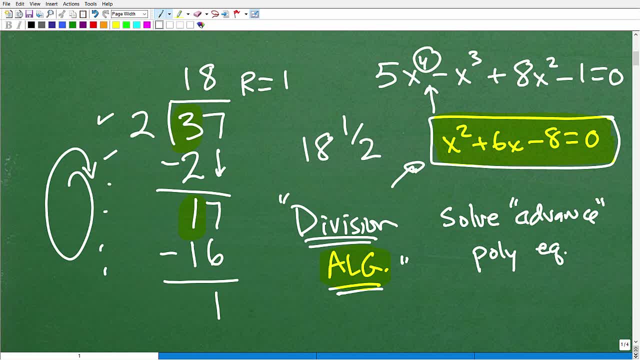 We could use a quadratic formula, et cetera, et cetera. So if you're interested about learning about quadratics, quadratic equations again, this would be like in my algebra two and algebra one course, But I have a ton of videos on this in my YouTube channel, in my algebra playlist as well. 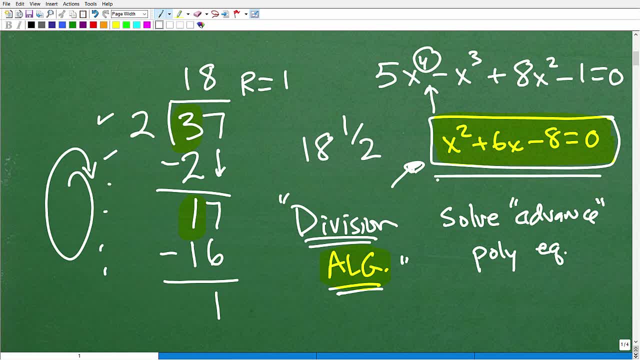 So you know most of you can solve this. Hopefully you've heard of quadratic equations, but we have tools and techniques to absolutely solve this equation. Now, when it comes to something above two, power of two like power of three, four, five. these guys. 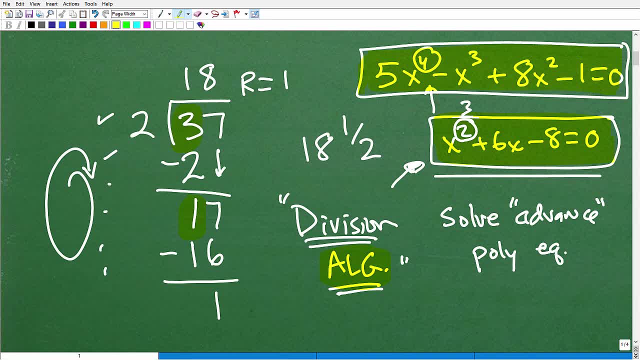 well, this is a whole different ballgame. This is where the real fun starts. It's in mathematics. So this is really what I would classify as more advanced polynomial equations. But guess what? They're equations too, and they deserve to be solved. 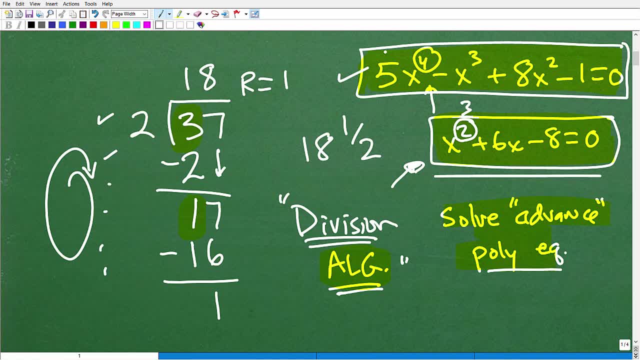 But we're going to need to use more powerful tools, And polynomial division is part of that new tool set, or set of tools that you need to solve these guys. We don't really need them over here because we have the quadratic formula, OK, so let's put this in context. 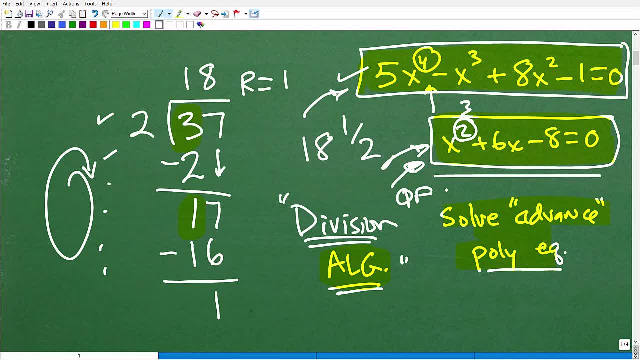 And when I have a title of like: hey, do you really need to know this? To pass algebra? I'm not lying, OK, I'm being very truthful here. All right, Let's get into this. And again, if you don't fully understand this, that's OK. 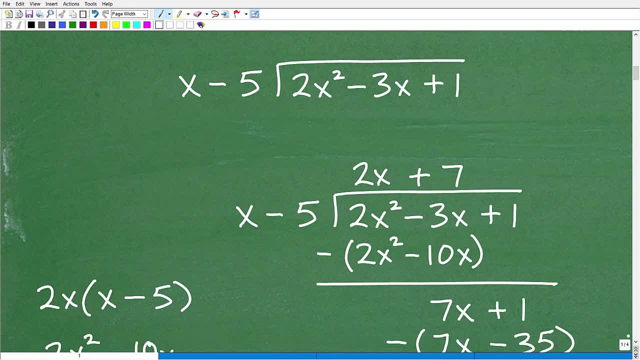 A lot of students don't. The first time, of course, you can watch this video again. I've done other videos on this in my YouTube channel, but I'm going to encourage you to check out my Algebra two course to really master this. 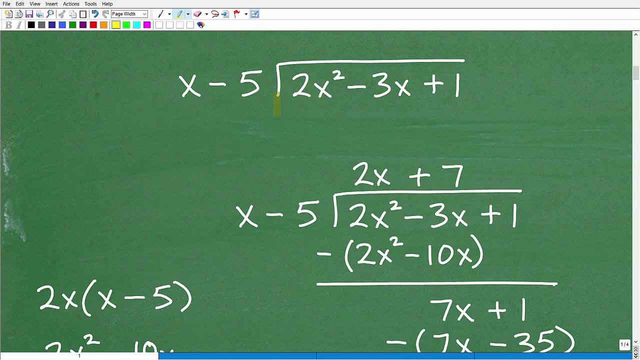 All right. Now here's our problem. OK, so we're going to divide this polynomial by this polynomial- And I'm specifically using this guy right here for a reason. OK, now this could be any two polynomials, OK, and this works exactly like when we're dividing numbers. 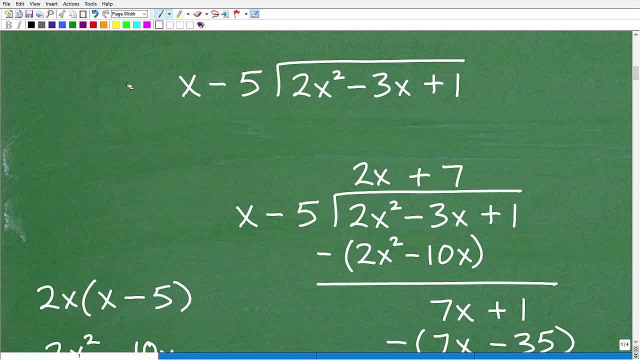 OK, we're going to be thinking the same way, All right, But here's how it goes, All right. So let's get started. You can see I've done some work here, So the first thing we're going to do- 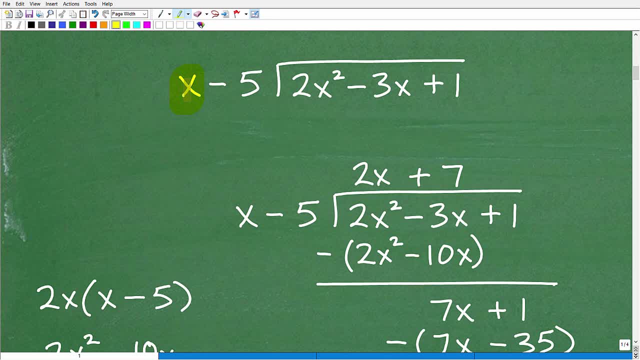 Is this. we're going to focus on the variable X. OK, We're going to focus on this part We don't really care about this other part will come into play. So I'm going to ask you: All right, What can I multiply this by this X to get to this here? 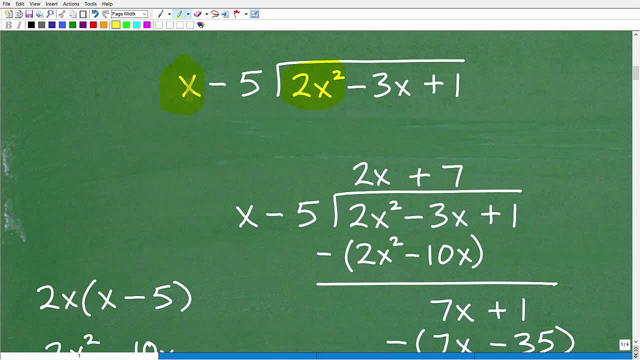 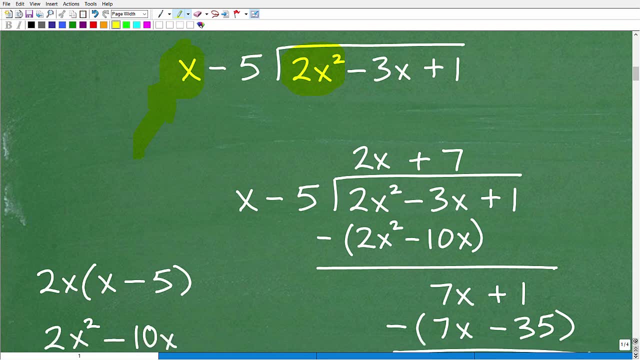 This number? OK, so what kind of what do I need to multiply this variable to get to two X squared Right? This is how you start these problems. So the answer is: well, what if we multiplied by two X? OK, so if I multiply two X by this X? 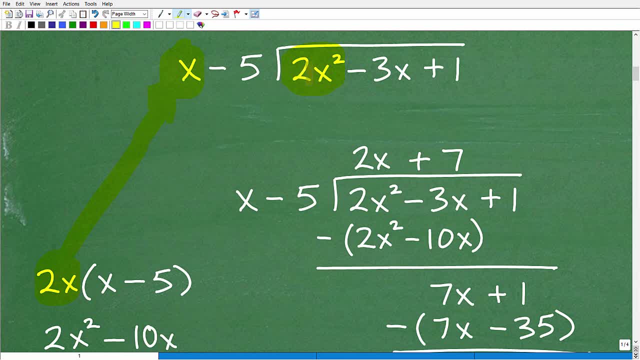 I would get to two X squared And that's correct. OK, so what we do is, once you determine what you need, to multiply this variable by this. In this case, it's two X. Now we're going to take that two X and I'm going to multiply. 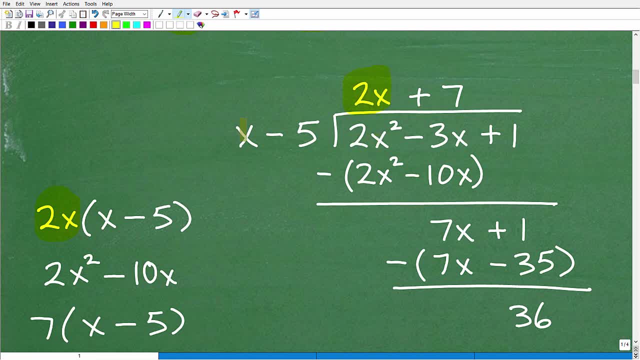 OK, it's two X is what I need to multiply X by to get here that I need to multiply X by two X to get to two X squared. OK. so again, I know it's probably a little confusing for those of you out there, but just keep watching. 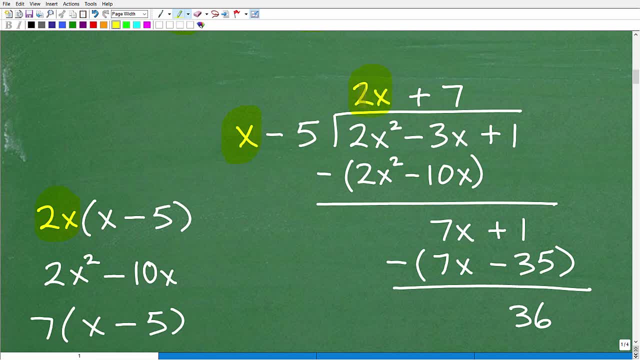 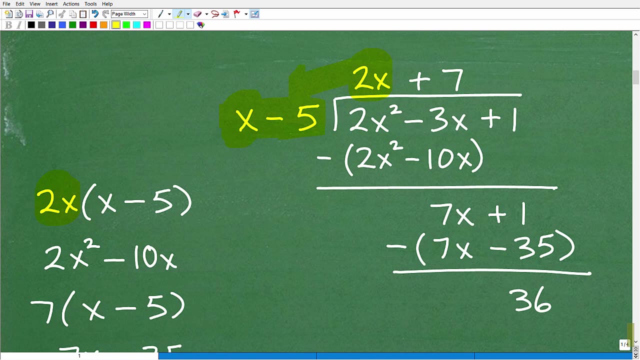 All right. So now that we determine that it's two X and I need to multiply this by, I'm going to multiply this two X by this whole thing here. OK, this follows what we were doing with arithmetic here. with that basic problem, I was at two divided in thirty seven, whatever it was. 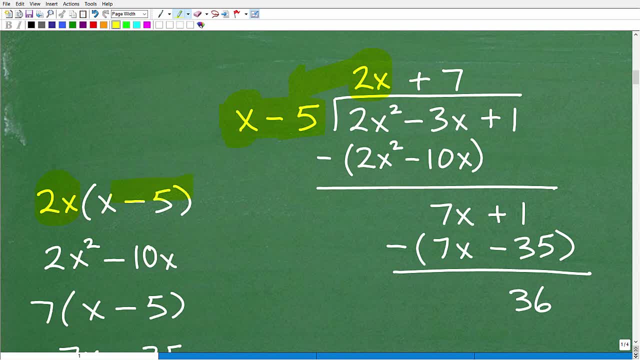 Right. So now we're going to take this two and we're going to multiply it by X minus five Boop, Just like this. So when I do that, I got to use the distributive property. So I get two X squared minus 10.. 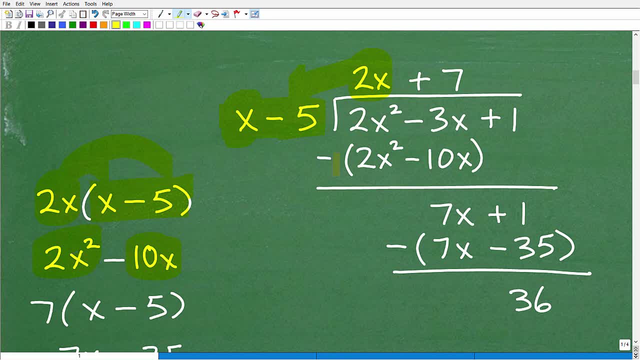 X. I'm like: OK, awesome, What do I do with that? Well, I'm going to subtract that from the polynomial. This is following the same steps as what we're doing with numbers. OK, let me go back up here. 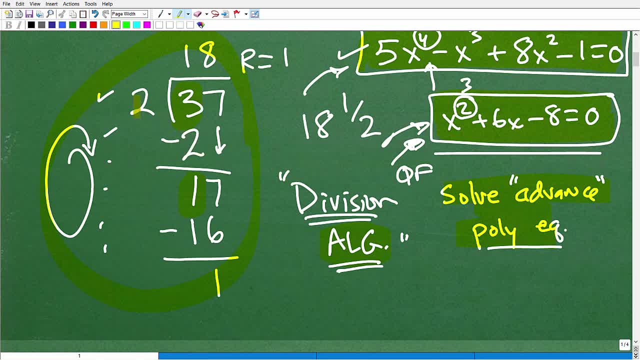 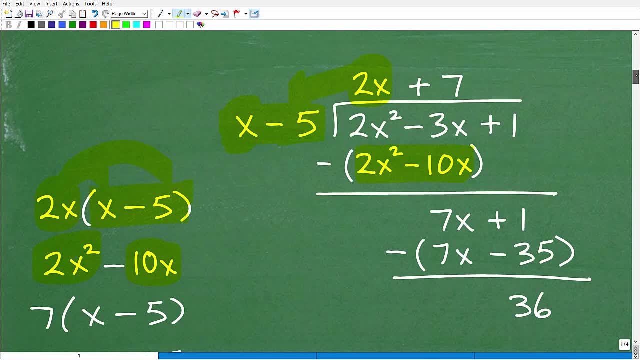 Right, here We're doing the same thing. OK, we're like: oh, what goes into this, What We're kind of effectively doing the same thing? OK, All right, So now let's go ahead and subtract, So distribute this negative. 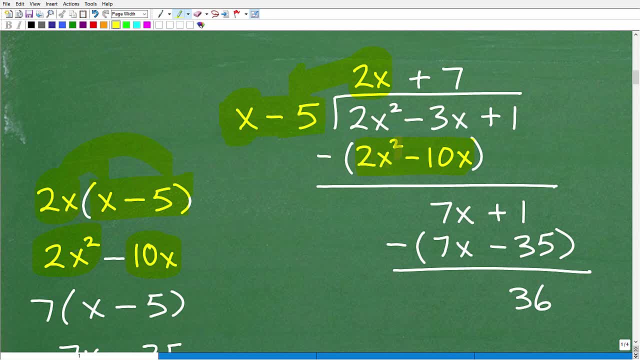 This becomes a negative. two X squared: This becomes a positive. This right here becomes positive. This becomes negative. And when I add down: OK, what happens? Well, the two X squared, these guys go away. This becomes zero, because it's positive. 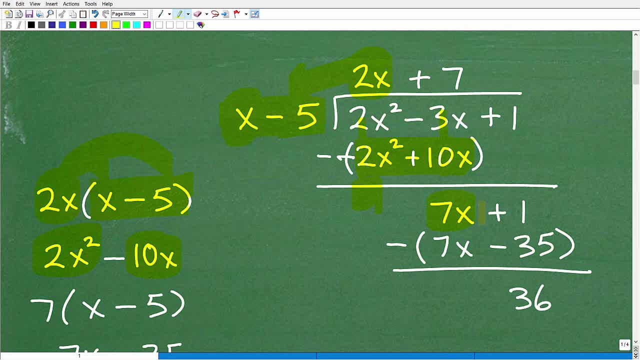 This becomes negative. This is positive, That's negative. So I get a seven X and then I'm going to drop down the remainder of the polynomial here. OK, All right. So if you understand what I just did, well, then all we're going to do that is the algorithm. 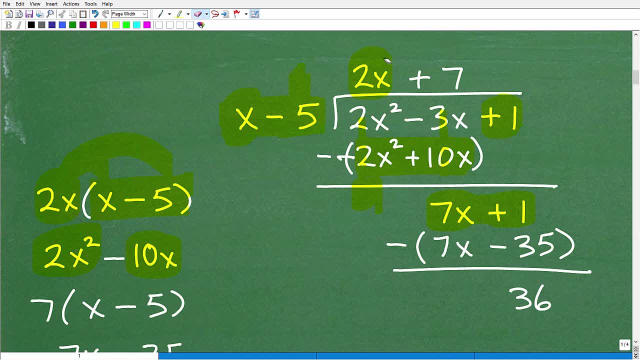 We're just going to repeat the algorithm. OK, so now let me go ahead and erase this stuff and we'll repeat the problem again. All right, So I got seven X now seven X plus one. So the question is the following: 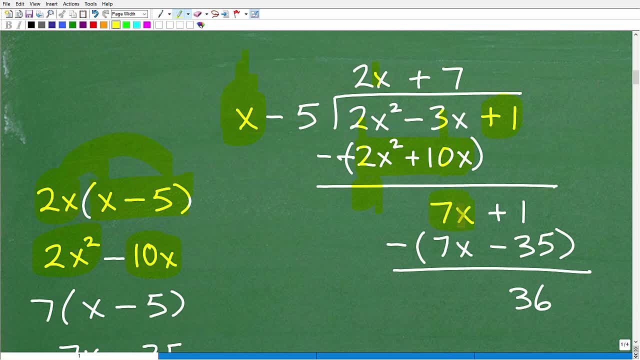 What do I need to multiply this X by right here to get to seven X? Well, the answer should be obvious: Seven. So seven times that X gets me seven X, and I'm going to multiply seven times this whole thing And I got that work right here. 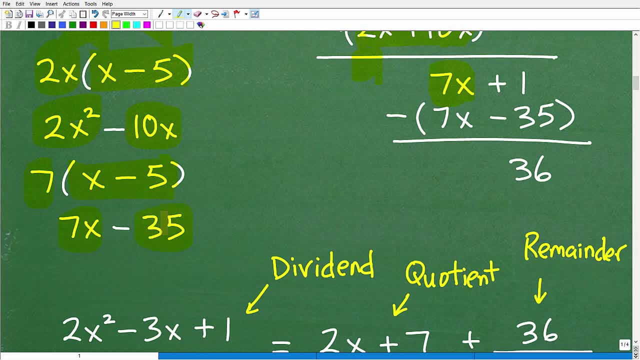 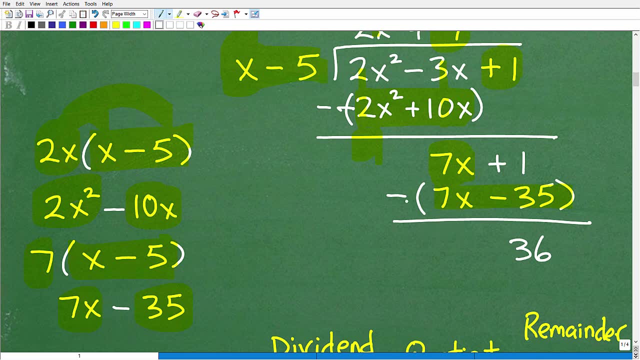 So seven times that whole thing gives me seven X minus thirty five. So I'm going to subtract that underneath here, just like this. We're going to do the same step. I'm going to distribute this. negative signs as becomes negative. This becomes positive. 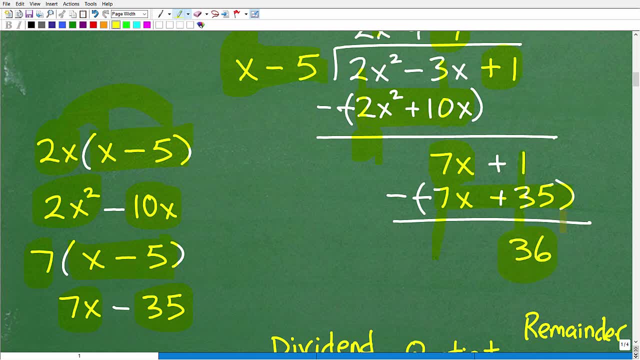 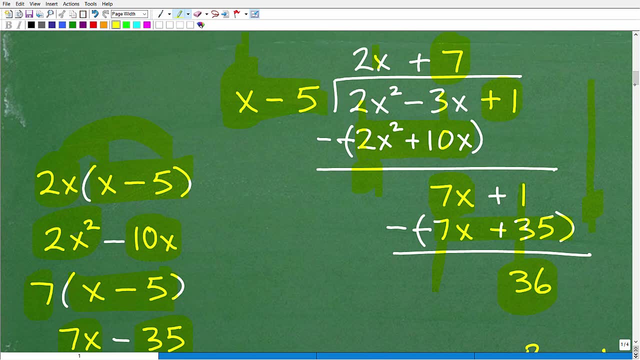 And then when I add down, OK, I get thirty six, and that is it, because I can't drop down, So X can't go under thirty six, And so you are done, OK. So you know, we've got to write this in a proper way. 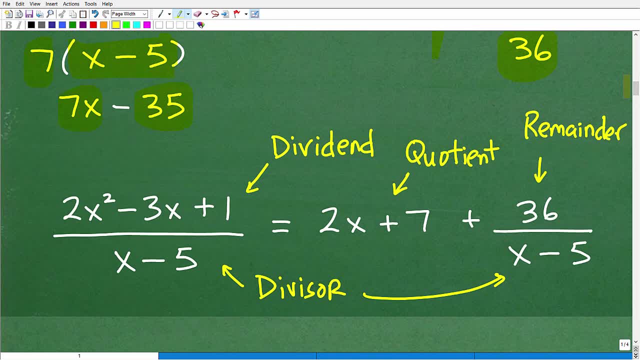 So let's recall some basic division terminology vocabulary. All right, So we did polynomial division. You can look at this way as well. Now, when you look at it in this manner, you're probably thinking of factoring, But this is division. 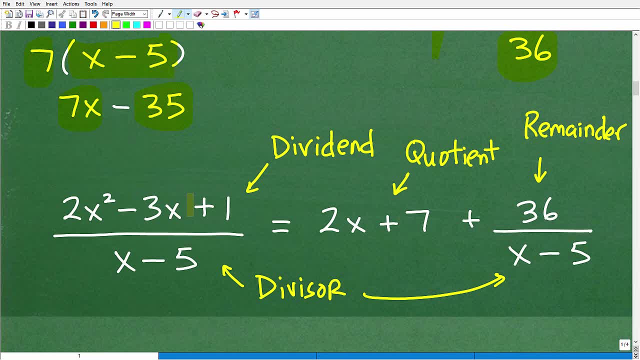 But it's really not. You know kind of the way you're thinking about. you're probably correctly so, looking at factoring and simplifying, but this part that we're dividing into, OK, that's called the dividend. OK, And this part down here is called the divisor. 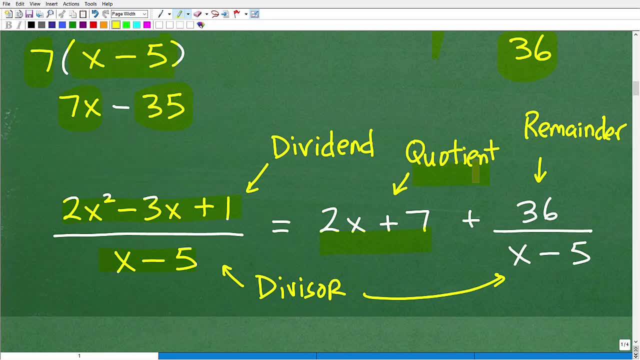 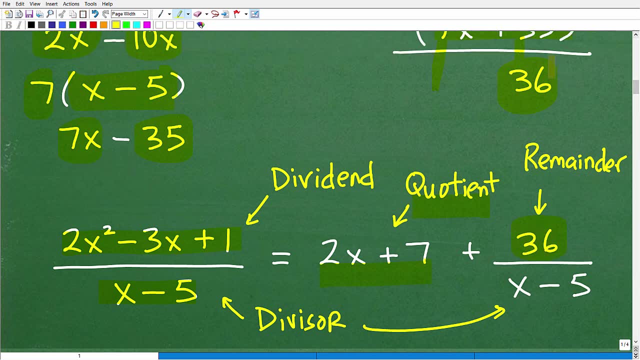 Then our answer is called the quotient. OK, that's the quotient. And then, when you write a remainder and polynomial long division, remember thirty six was our remainder right here. OK, remember our, our last part of our answer. That's the remainder. 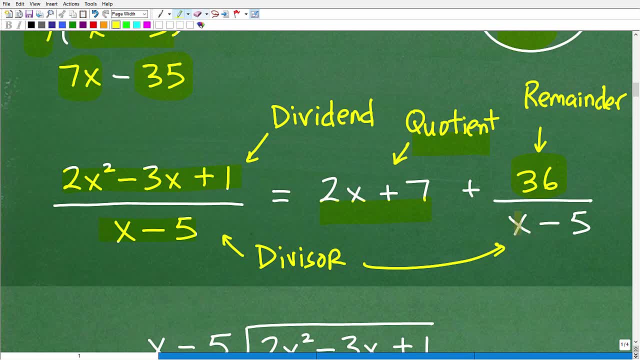 But you write it over the divisor like this, as a fraction: OK, so this is an introduction polynomial- excuse me, polynomial, a long division right now. Again, I know I'm covering a lot in a short period of time, but this is important stuff. 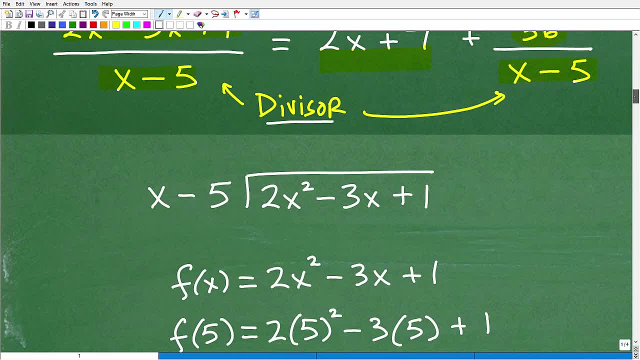 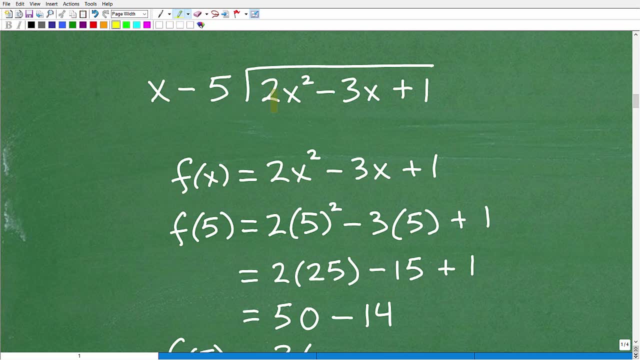 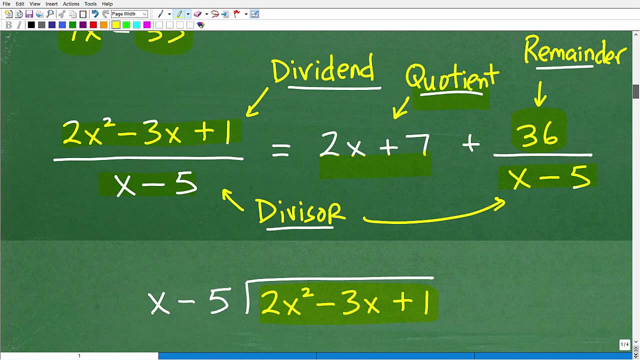 Now let's go ahead and do something very interesting here. OK, this is, this is really the value of why you want to learn this. So here let's take a look at this part of the problem, which, of course, is called the what, the dividend. 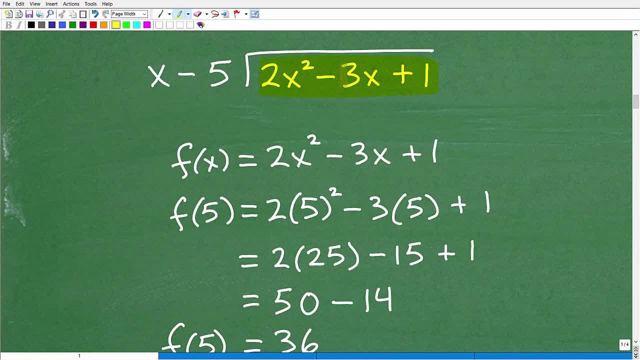 All right, Then we have the divisor, But let's just focus on this, OK, so here is this part of the problem. Let's write this as a function. OK, you're like: well, where are you going with this? 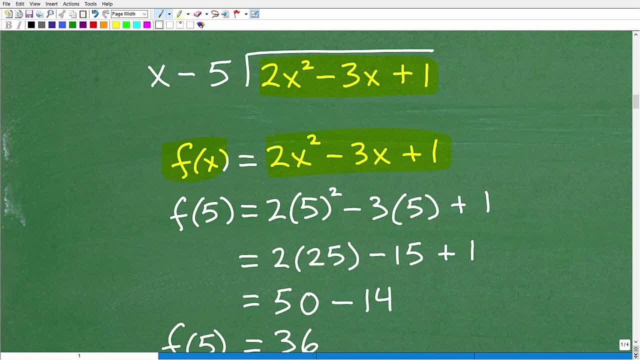 Well, I'm going to show you this here, precisely because this is really why we're studying this. So I got X minus five and I'm dividing it into this polynomial. Now let's evaluate this function right here for five. OK, what does that mean? 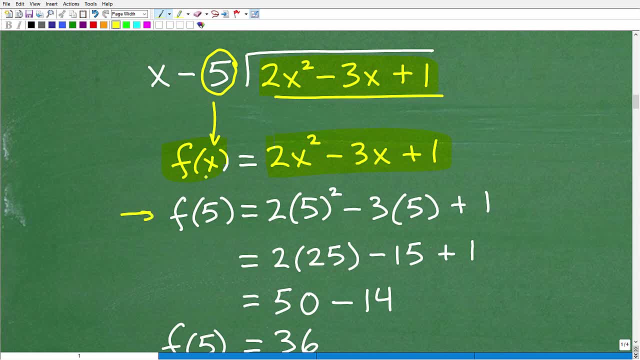 Well, I want to find F of five. That's what it means. I'm plugging in five into the function, You understand? OK, All right, So hopefully do. Let's go on and do the work- And obviously I've already done it here for us. 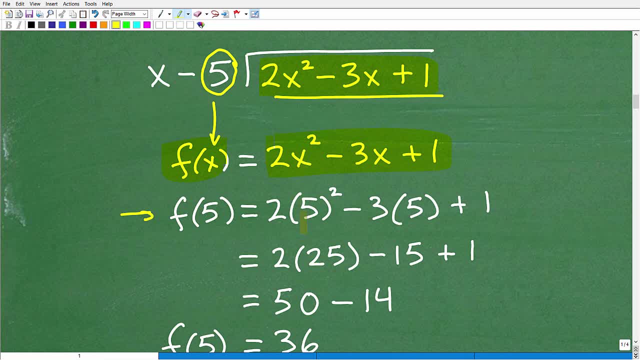 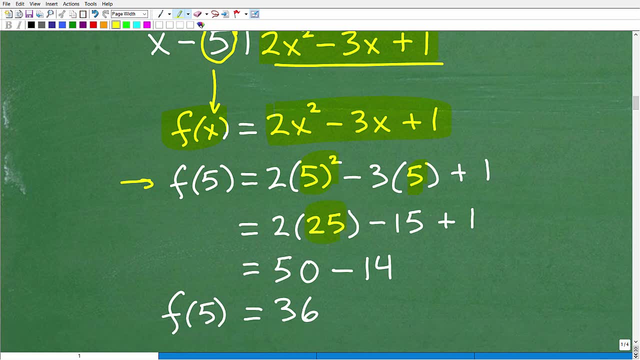 So when we find F of five, we plug in five for X, just like this: Wherever there's X, we're going to plug in five. And when I do all this I get what? Five square, That's twenty five. 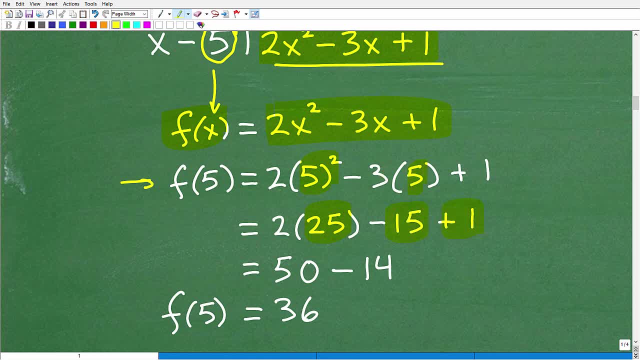 This becomes three times five, That's a negative fifteen plus one. Two times twenty five is fifty, So this is a negative fifteen plus one, That's negative fourteen. So fifteen minus fourteen is thirty six, So F of five is thirty six. 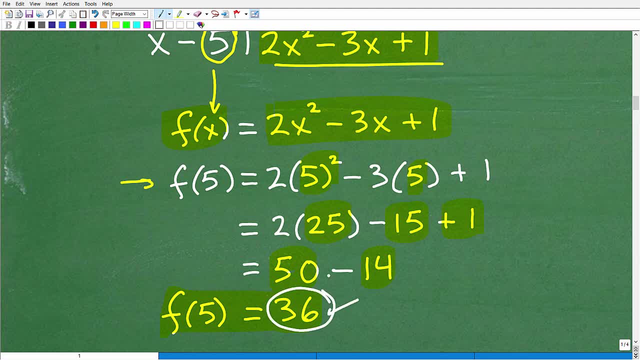 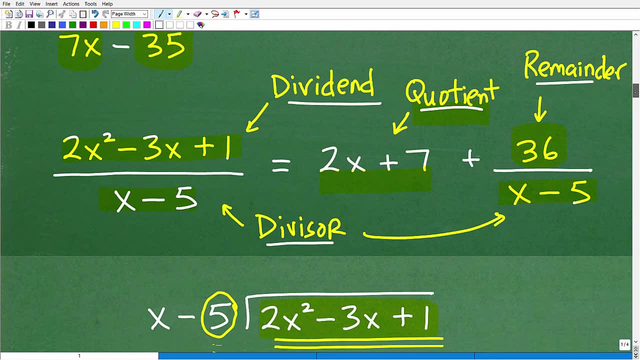 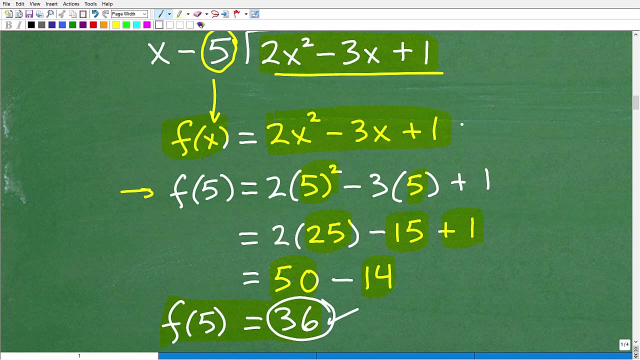 Hmm, How interesting, Doesn't this number ring a bell? Well, it happens to be the remainder over here. OK, so there is a connection to this. So you're like, oh, that was interesting. So I evaluated this function for five and I got thirty six. 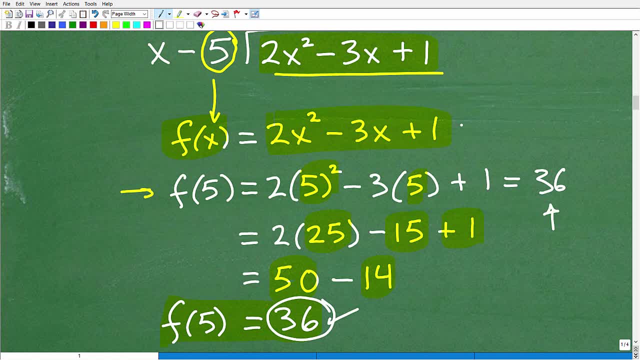 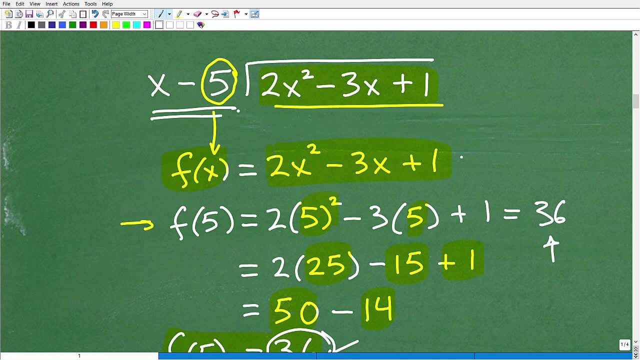 which is happens to be the remainder. if I divide by five, OK, we're polynomial. where this is five, OK, and now this is called a linear factor. Now, this is just an overview of this stuff. I'm sure I'm trying to make these connections. 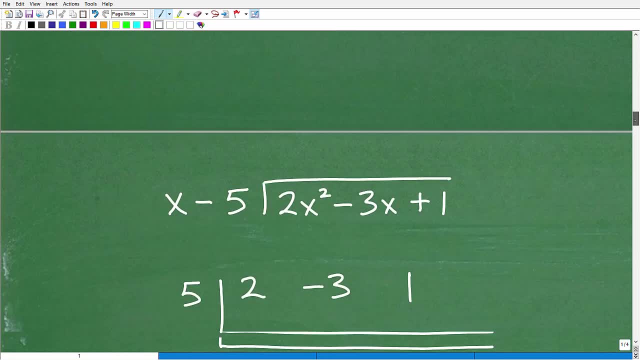 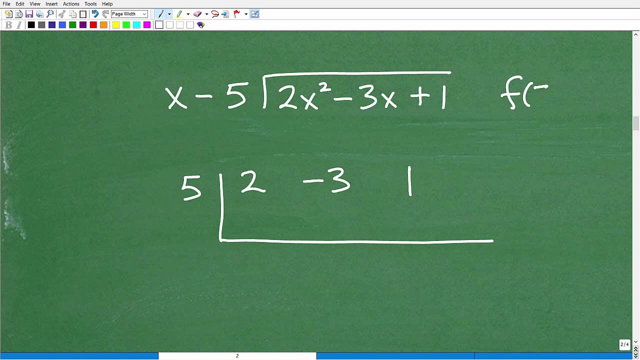 Now I'm going to show you another way to do this, And this is super cool. All right, Now what I want to do here is I want to find F of five of this function. OK, Now, this the way this is written, this number when you have an X. 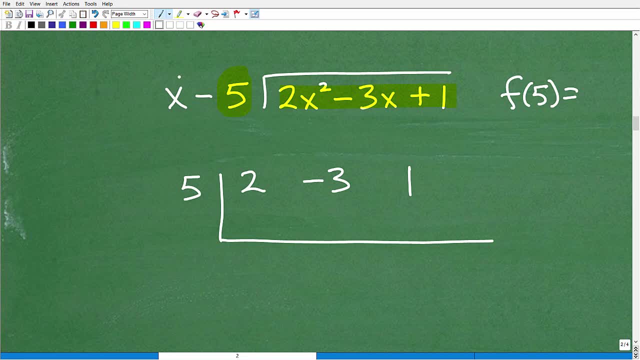 OK, it's specifically an X, not an X squared, It's an X. All right, Let me show you this right here: X minus could be anything, could be seven If you're dividing into a polynomial, and it's X minus. whatever this number is. 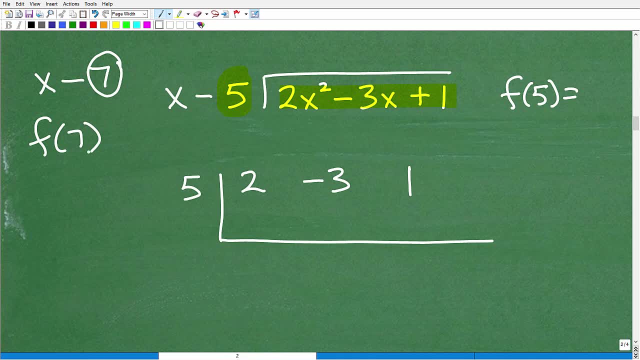 it's the same thing as evaluating that polynomial for that number. All right, Now what about if I had X plus three? Well, we have to write this as X minus minus three. So X plus three. If this was, if this was, an X plus three, right here. 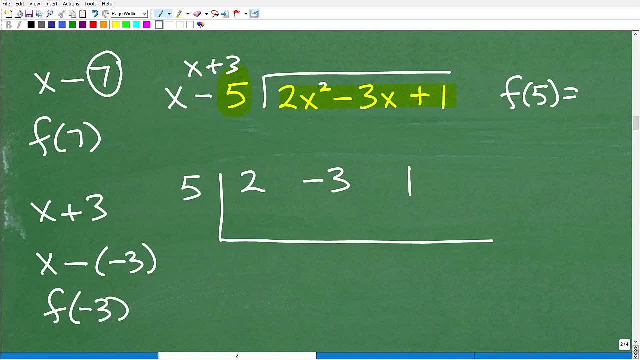 this would be the same thing as F evaluating the function for F minus three. This is extremely important, So hopefully you kind of get the essence of what I'm talking about. But in this case I already have F minus this number. I'm sorry, X minus this number. 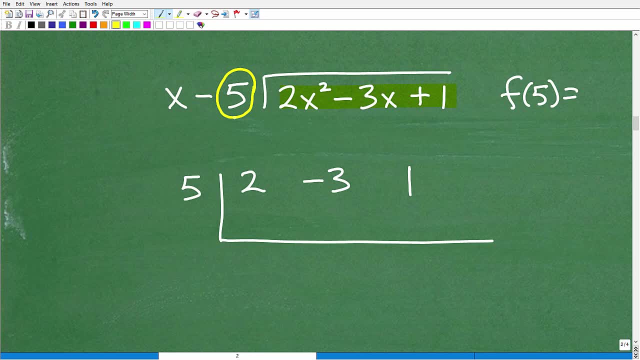 So this is the, the value. that is basically. I'm going to evaluate this value right here into this function. So what I'm going to be doing here is the same thing is as finding F of five. Now, remember, I just found F of five. 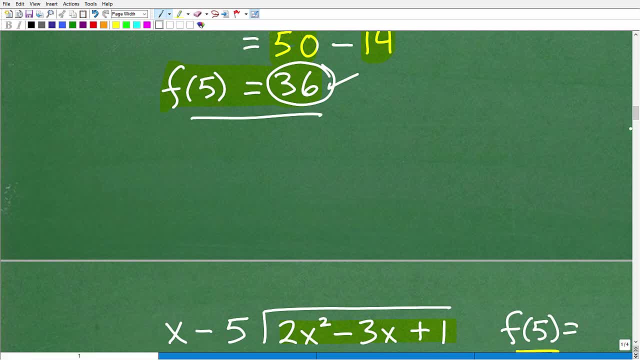 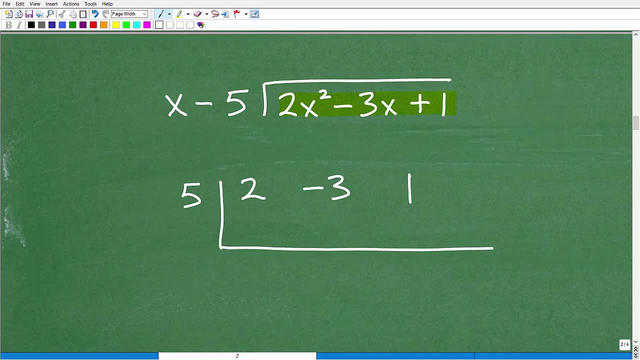 All right, What does F of five equal to? F of five is equal to thirty six. I'm doing this problem, but now I'm doing this using something called synthetic division, which is totally awesome. It is like it's, and it's actually fun to do. 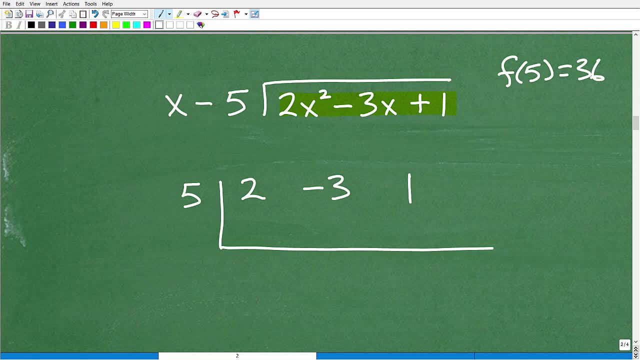 Some of you might think, OK, this guy is definitely crazy, but it is really, really Shortcut, All right. I mean, if you're looking for shortcuts to math, this is one of them, right, All right. So how does this work? 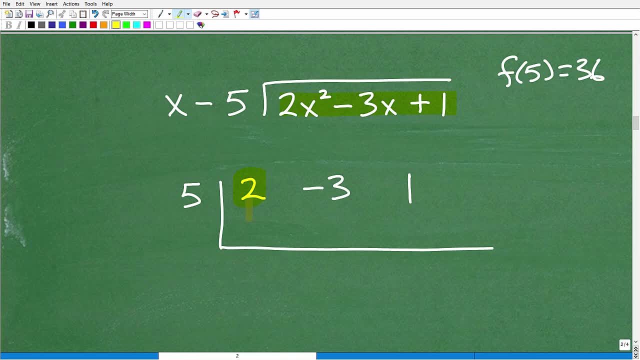 Well, it's super easy. What we're going to do is going to take this number two. We're going to plop it down right here. We're just drop it. We're going to write it to you like that. OK, so here we go. 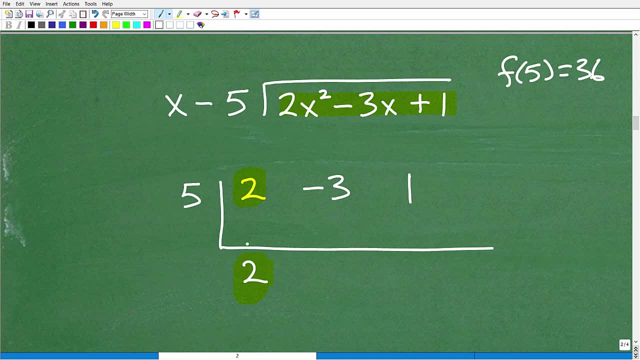 And now this is a little algorithm. It's called synthetic division. So we're going to take five times two. Five times two is what That's ten. All right, Now we're going to add down. OK, we're going to write our answer. 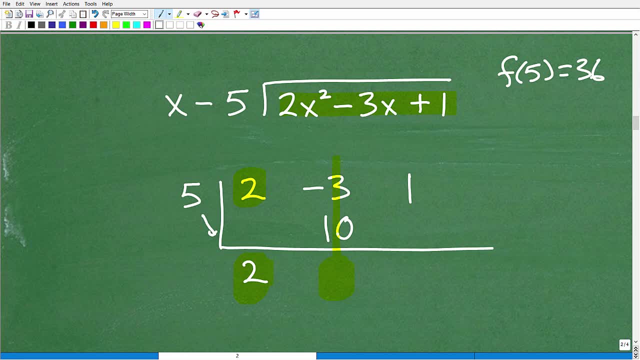 Right here. we're adding: So negative three plus ten is what Seven? OK, we'll do this again. So it's going to be five times seven. We're going to put our answer right there. What's five times seven? Last I checked, it's thirty five. 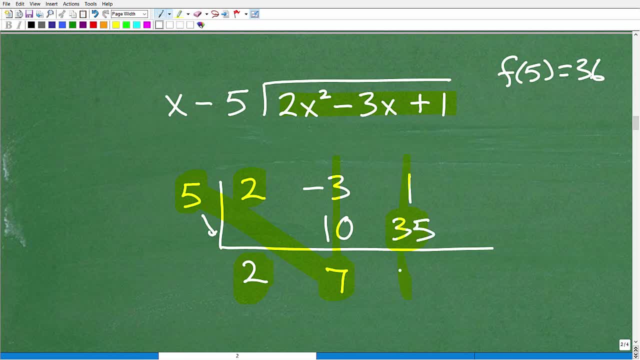 And then we're going to add down And what do we get? Thirty six, This last spot when we do this, this is the remainder, OK, and it's thirty six, OK. this is the same thing. So You do synthetic division when you plug in this number. 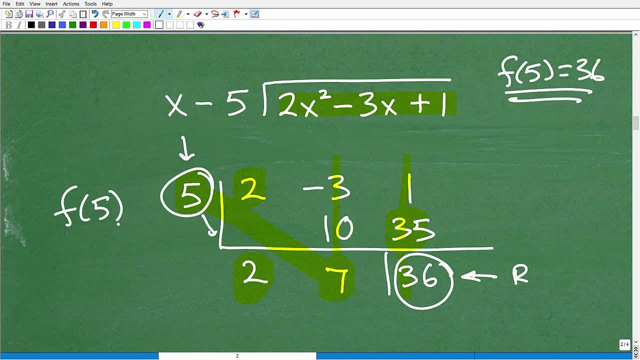 It's like, basically, you're going into the function, You're saying: what is F of five? equal to it, Whatever, whatever the remainder is equal to. whatever the remainder is is what F of five is equal to. So F of five is equal to thirty six. 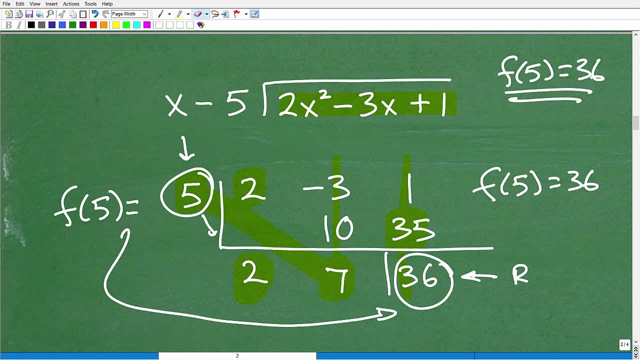 But look how fast I was able to do this. OK, I could plug in any number here to quickly evaluate this function. OK, now what you're really looking at is zeros. All right, This is a whole other discussion, and that can go on and, on, and on. 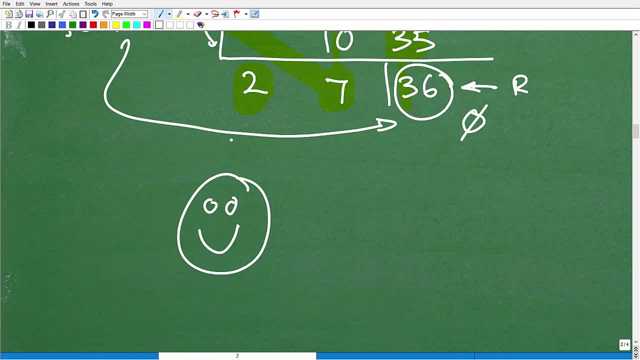 But hopefully you're pretty impressed with that. Hopefully you're like: wow, that is so cool. OK, by the way, if you knew this, then I must, you know, give you a large Mohawk, like we used to have back in the good old 1980s. 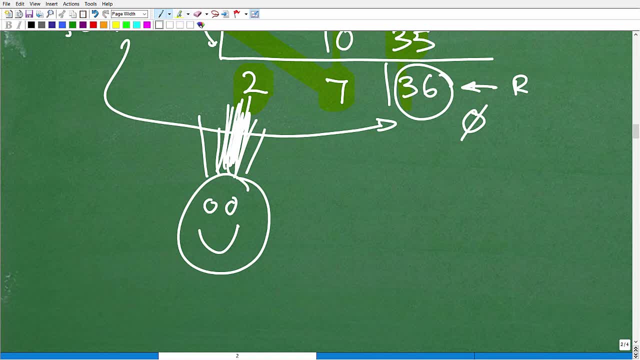 We used to use a lot of hairspray. I think some of you who watch my videos maybe I've said that before. It's probably pretty dangerous to have that much hairspray in your hair. But anyways, if you knew this and you knew all of this, 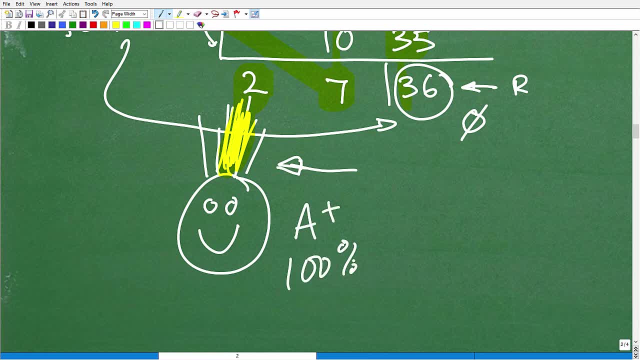 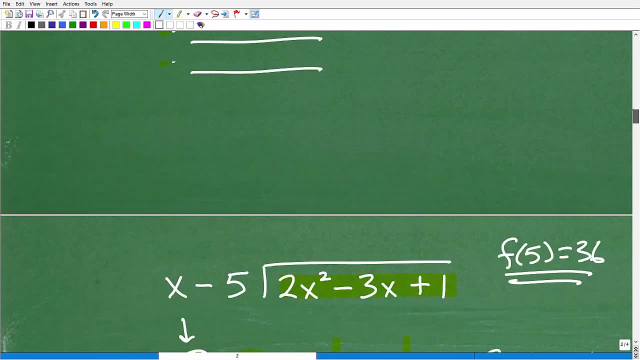 and I'm pretty sure you're tracking for a plus one hundred percent Matter of fact, if I was your teacher I'd say: you know what, just go home and I'll see you next year, because you're obviously doing all the right things. 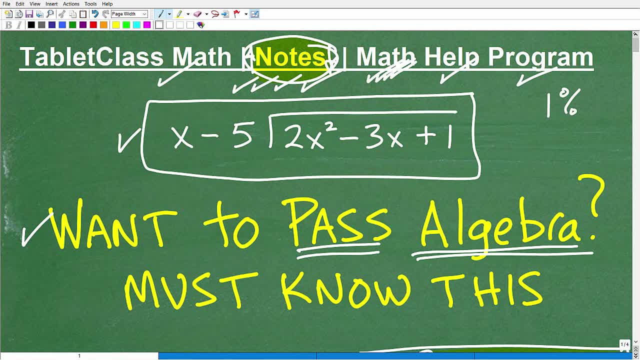 You're probably watching that guy on YouTube, But anyways, listen, here's the bottom line. You need to understand this. I know it's a little complicated and this video, hopefully, was a good introduction, but it by no means is a complete full lesson that covers everything you need to know. 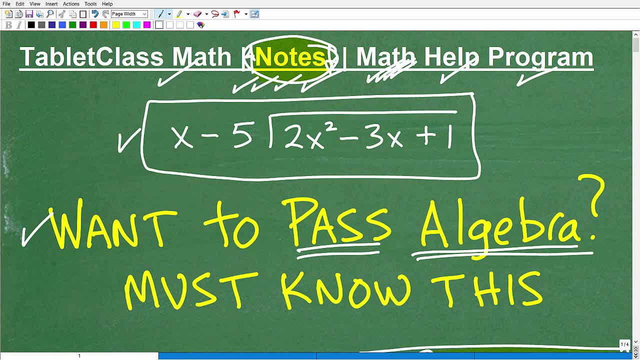 About this. This is stuff you're going to have to practice. So again a couple of suggestions. One: I have additional videos on polynomial long division on my YouTube channel or my- I think my- Algebra two playlist, But my best math help on this would be: 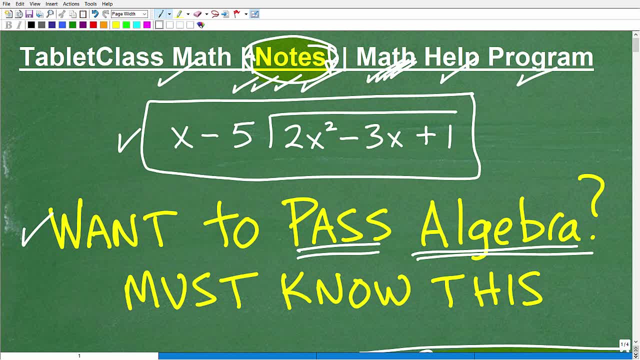 within, like my Algebra, two course that you know you might want to check out. But if this video was interesting and you actually liked it, OK. if you did like it, well, that's awesome. Please consider smashing that like button and please consider. 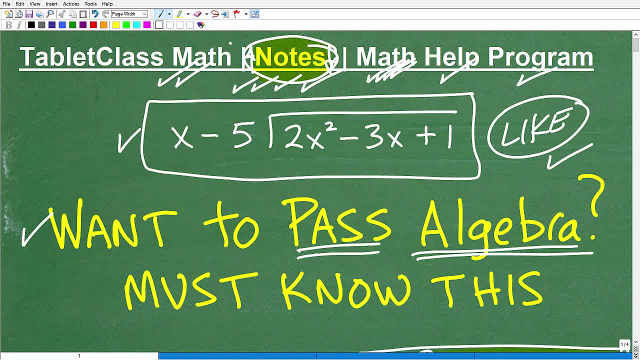 subscribing. I've been on YouTube for ten plus years. I have over a thousand plus videos And, if you like my teaching style, all those videos are there for you. I make these videos so people can watch them and learn math. My passion is to try to make math clear and understandable.